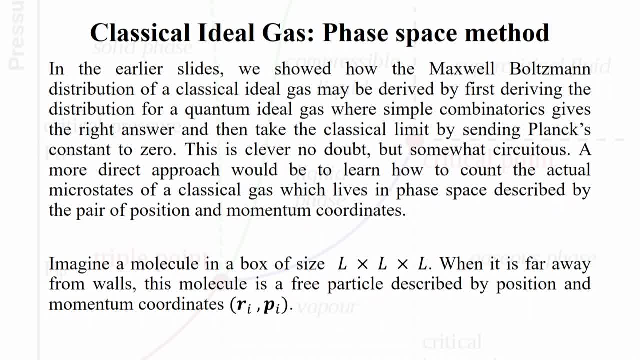 to do is we have to populate that phase space by all the n classical molecules that we have in our possession in such a way that we force those molecules to occupy a certain restricted volume. So let us say we talk about a cubical box of side L, So you have a cubical box of side. 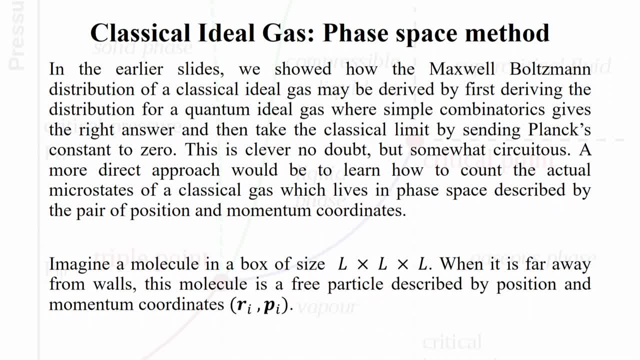 L by L by L, and I force my molecules to be present only in that box And I also make sure that, importantly, the other constraint is that I have to make sure that the total energy of all the molecules put together is some fixed quantity. So notice that when I talk about energy I only talk about kinetic energy, because I am 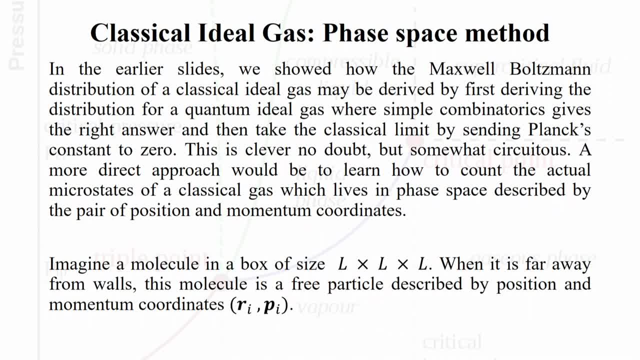 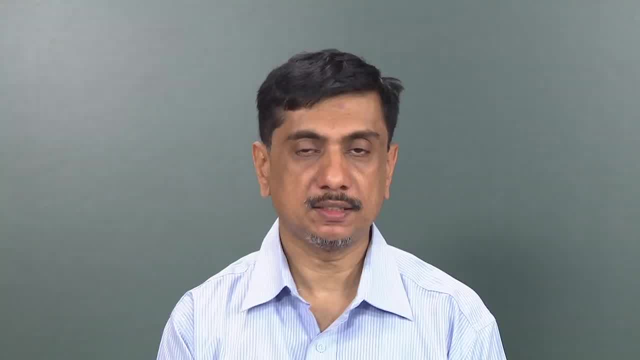 talking about an ionic energy. I am talking about an ionic energy, I am talking about an ideal classical gas. So they do not interact with each other except, you know, perhaps with the walls of the container. So until hit the walls of the container, no forces. 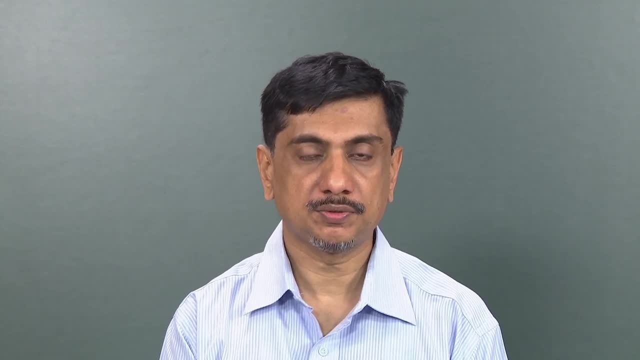 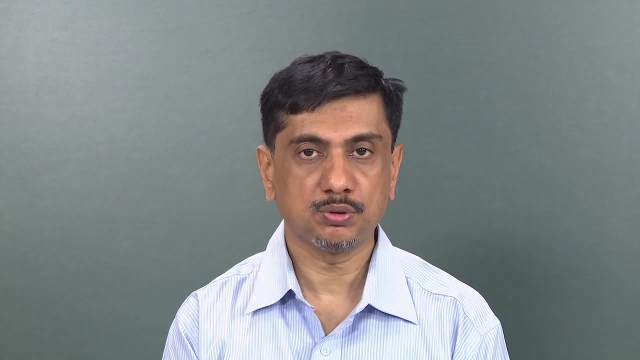 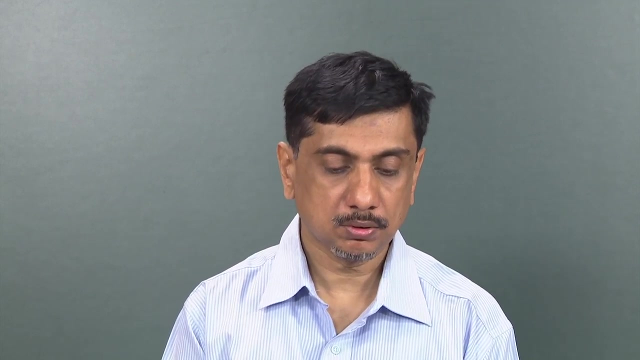 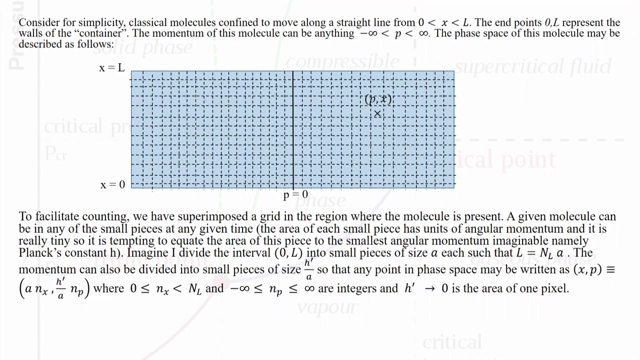 act on them. So within the walls of the container. so it is just kinetic energy of the particles. So just by forcing myself to only consider particles that live inside the container, I can be sure I am not making a mistake. So I would think the count when the object that I want to count is not discrete but some. 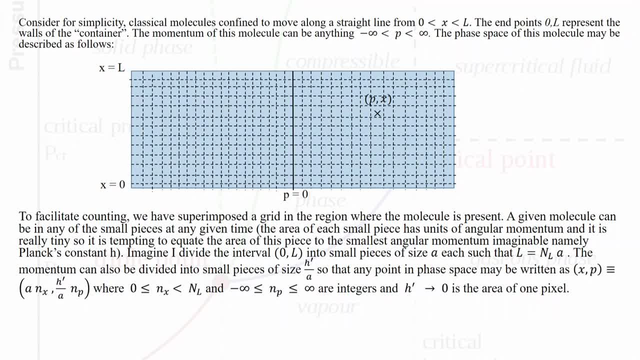 continuous. So it is. it is somewhat like you know, if somebody asks you to count the number of water droplets in the ocean, you would probably laugh at that person and say: well, ocean is just one continuous body of fluid. I cannot really count the number of. 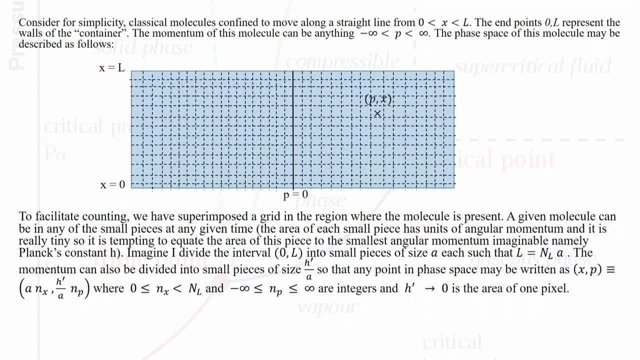 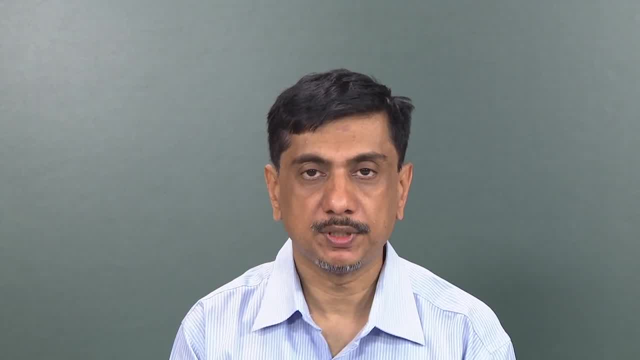 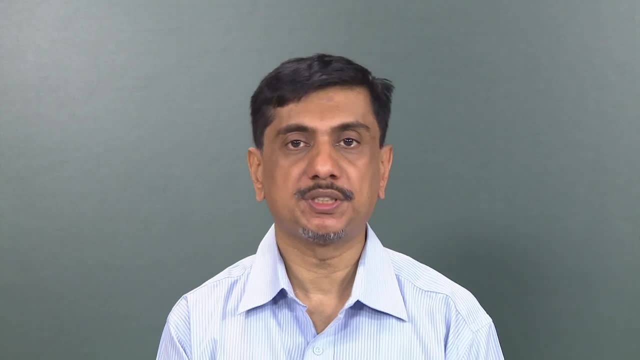 what does that even mean? So that is the problem we are confronted with right now, because we are being called upon to count the number of, you know, points, as it were, in phase space, when in fact the phase space itself is described by position and momentum, and or the components. 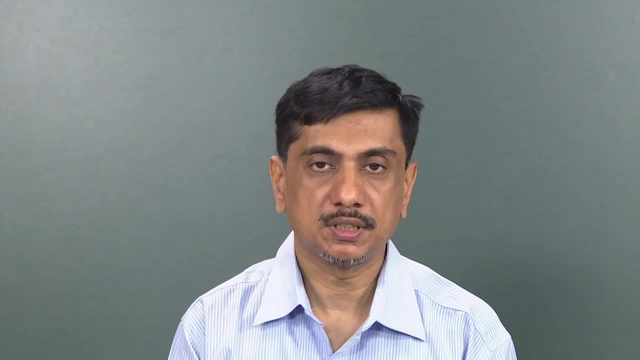 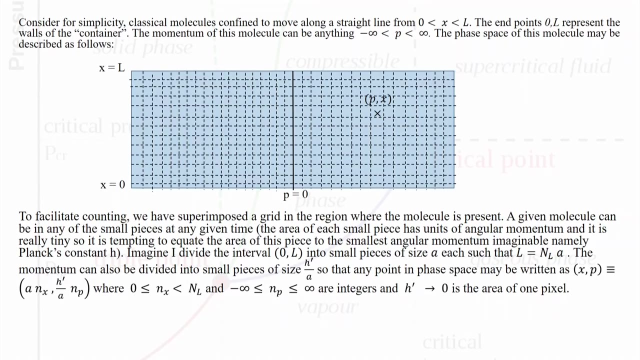 of position and momentum, which are all continuous, and so there is no way of counting a priori. So what we do in order to facilitate this is that we discretize. we artificially divide up the phase space into small pixels, So it is similar to what you have on your computer screen. 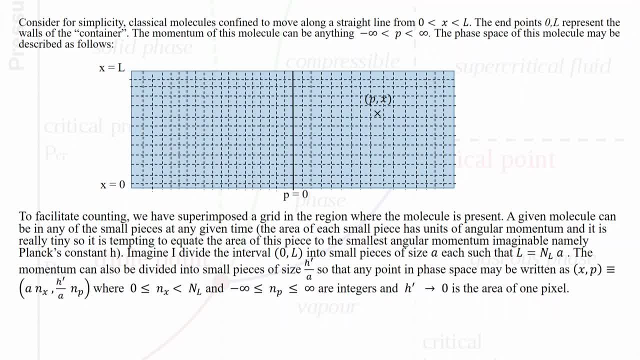 Your computer screen does not look granular, so it looks rather smooth and continuous. but then if you look under a microscope or a lens you will see that it is actually made of pixels. So pixels are small squares. Each square has a uniform intensity of a certain color. 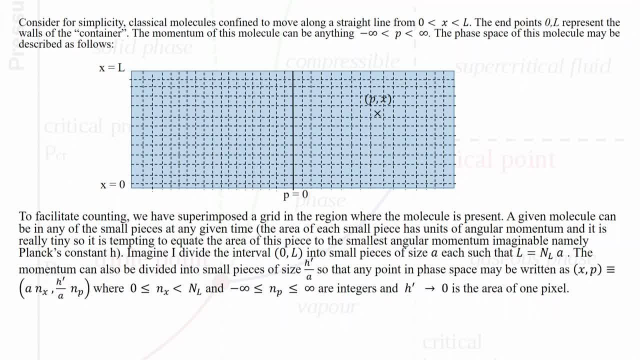 So we are going to do the same thing here. So we are going to take this phase space out here. So I have purposely restricted myself to molecules moving in one dimension. So, in other words, my molecules are forced to live between x equal to 0 and x equal to. 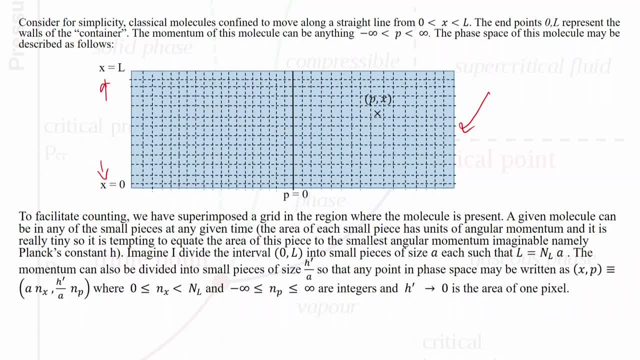 L and, however, they are not restricted to any particular momentum. They can have any positive momentum, However large, Or any negative momentum, implying that they are moving in the opposite direction, Also, however large. So I have this rectangularish looking phase space and I want to populate this phase space. 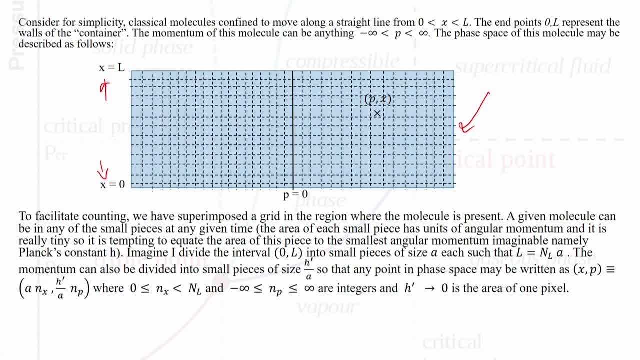 with my molecules. but before I do that, I have to. in order to facilitate counting, I am going to discretize this phase space by imposing a certain grid on it, which is basically same as dividing it up into a whole bunch of pixels. So how do I do that? 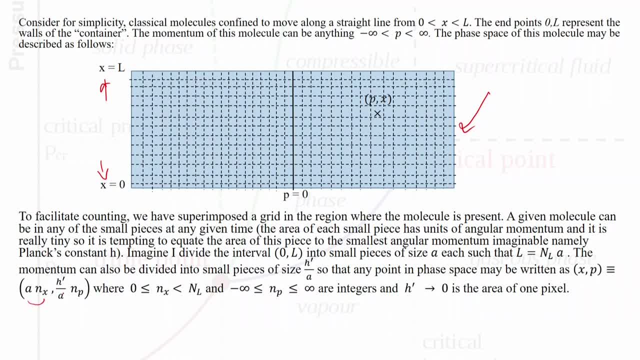 I say that. imagine that the position which is this axis, I should have flipped these 2 coordinates. So I am talking about the position here. So the position is this is x. So I am going to call n x. I have defined n x to be x by a. 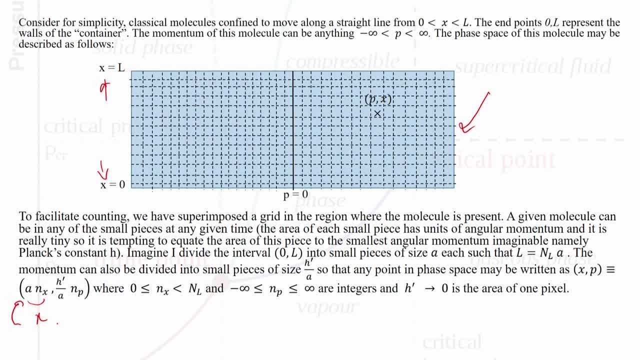 So, in other words, I am going to say that x is some kind of a multiple of a small number called a. So, in other words, I am dividing up this interval from x equal to 0 to x. So this is x, So this is x. 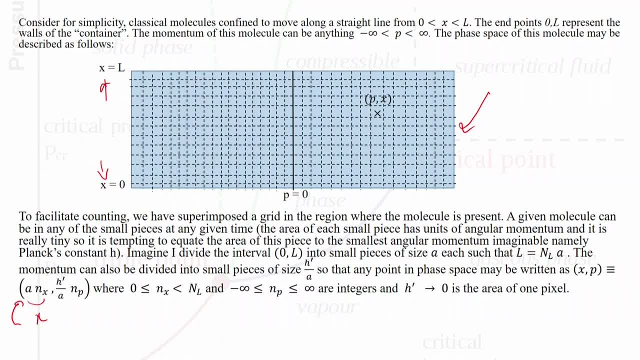 X, equal to L, into a whole bunch of pieces, and each piece has a size or length, A. So, and NX would be the number of steps I have to move in this direction in order to reach X. So, similarly, I do the same thing with P, except that I want to make sure that my, the 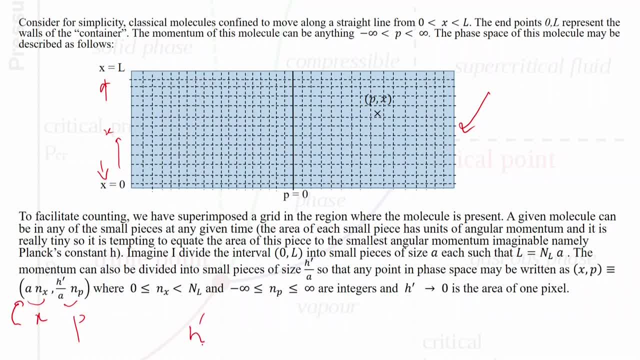 size of my pixel is some quantity. I call H H dash, So right now it has no special significance. later you will see that it is indeed very special, So we are going to discuss that later. Right now it is just a. you know, the area of my pixel which I have mandated, or by Fiat. 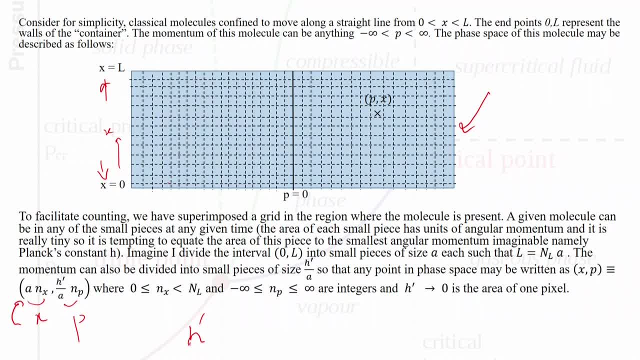 I have chosen it to be H dash. It is just a notation for a pixel of a small size. So because the pixel area is H dash, I will be forced to express my momentum in terms of discrete multiples of H dash by A, So that if I take the product of the length and the 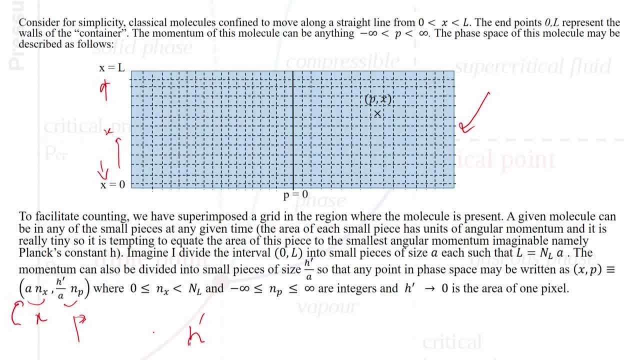 breadth Of the pixel, I get H, dash. and NP is an integer which can be as negative or as positive as it wants, and, however, NX. because my Xs are all positive from 0 to L, I am forced to choose my NX to be between 0 and a maximum value determined by, of course, this NL would be nothing. 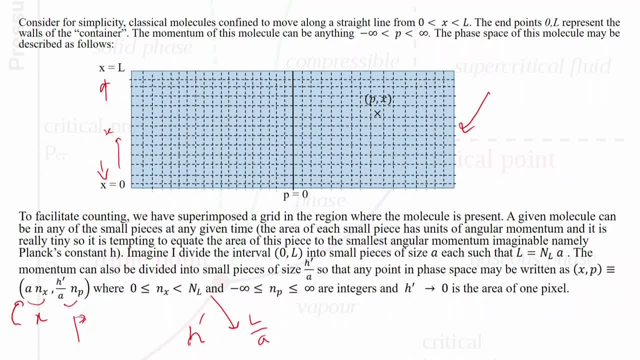 but L over A, where L is my, the size of my system, the physical size of my system divided by the size of each pixel, The X size of each pixel. So of course, I mean you might be wondering what gives me the right to do this, because after all, it is a very contrived and artificial thing to 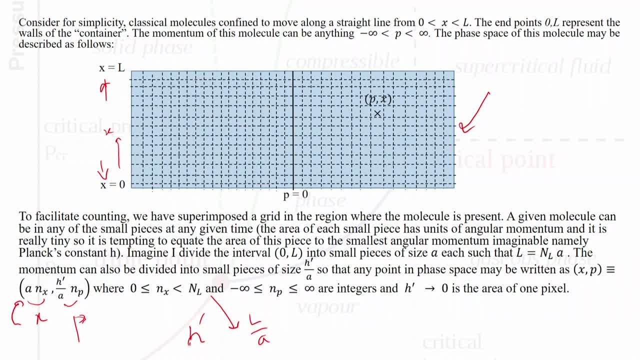 do and of course implication is that towards the end I am going to make the pixel size tends to 0. So I am going to make the pixel go away and everything becomes nice and smooth and hopefully I will be able to stack the pixels October. 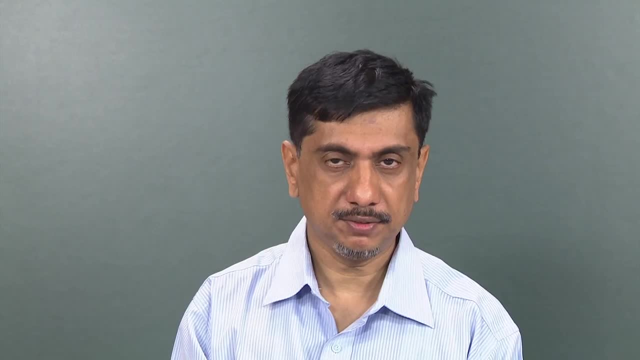 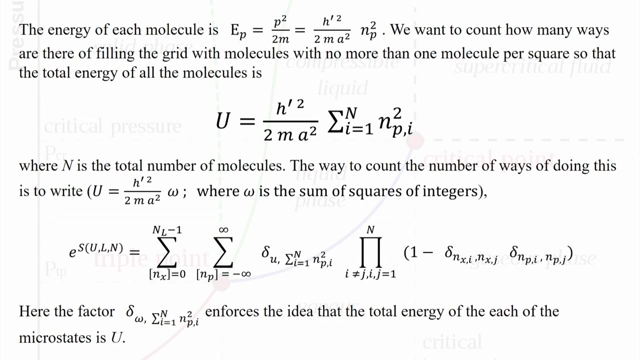 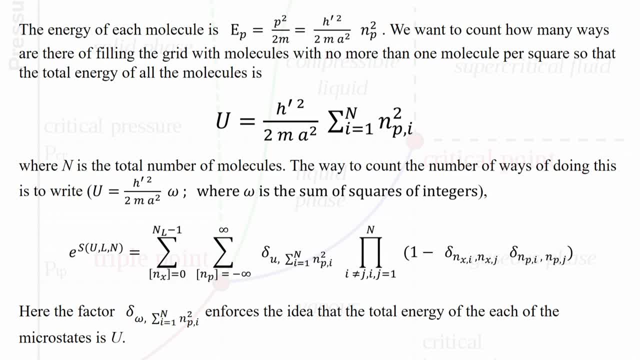 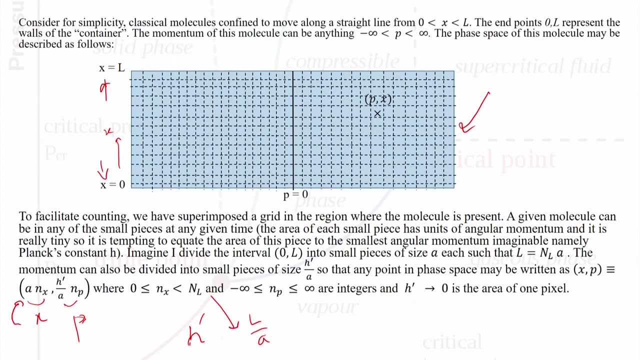 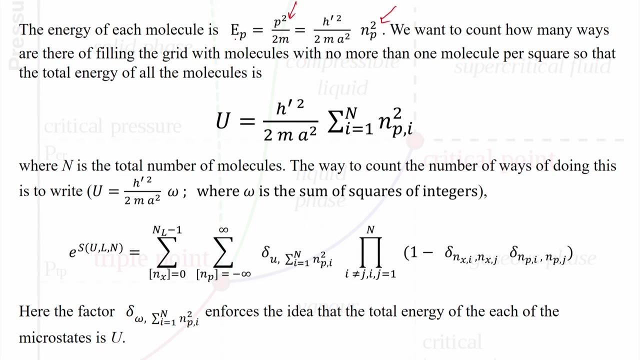 numbers called Nx and Np. okay, So how do I achieve that? So I simply know that the energy of each molecule with momentum p is p squared by 2m. So I can rewrite p in terms of Np here, and so if I do that, I get this quantity here. So the energy of each molecule is proportional. 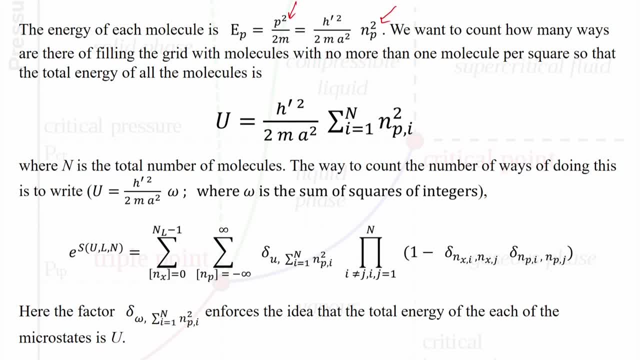 to that square of that integer. So notice that I have to ensure, in addition to, of course, ensuring that the particle does not exit my system. in other words, its position is locked between x equal to 0 to x equal to L. I have to make sure that it also all the molecules. 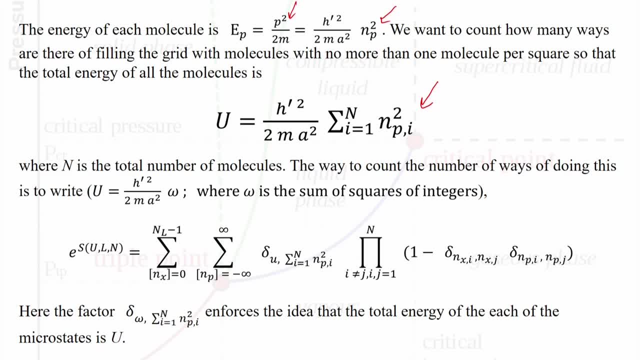 put together should not have any energy other than p. So in other words, its total energy of all the molecules put together is forced to be u. So notice that this index- I refers to the index which tells you which molecule I am looking at. So if I equals 1, I am looking at the first molecule. if I am looking at I, 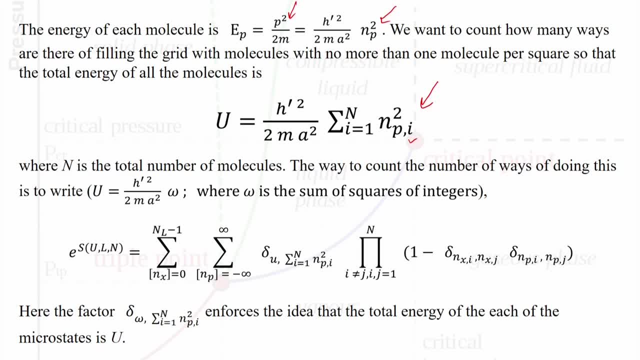 equal to 2 is the second molecule, and so on. So, and capital N is the total number of molecules. So when I do this, if I fix u so as usual, I have a kind of Diophantine type of system, so where I am being forced to find out all the different u's that are possible, which? 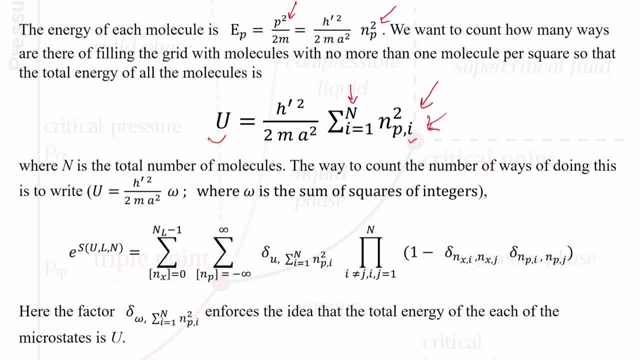 ensure that the total energy is u. So naturally, I am tempted to rescale or redefine my? u in terms of this dimensionless energy called omega, So which happens to be an integer, because, after all, it is just the sum of the squares of integers. So this also had better be an. 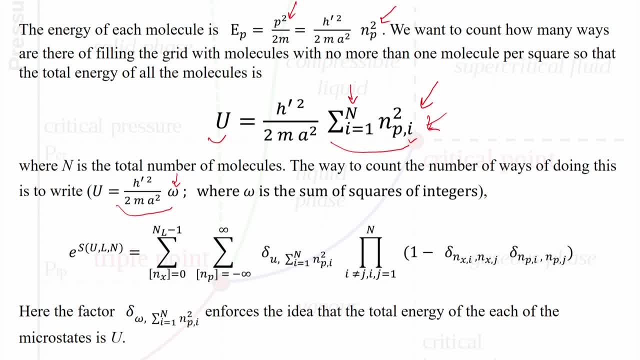 integer. not only that, it is the sum of squares of certain class, certain set of integers. Okay, I had to recall this. u not u, but omega. I called it omega because notice that I have reserved the symbol u for u by N and because of that I was forced to call u by V as using. 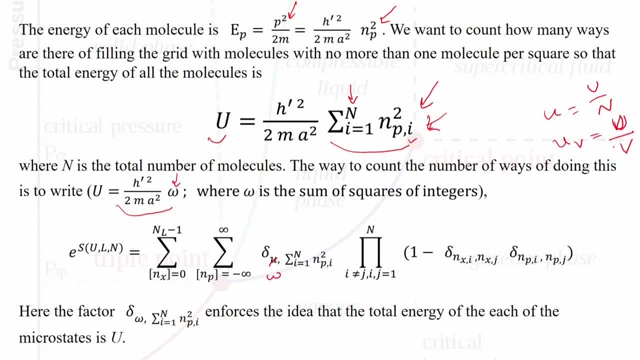 a different name, so I was forced to call u by V, as small u with the subscript capital v. So I do not want to confuse my listeners, So I am going to make this conventions to standard right now. So the small case u is nothing but total energy per particle and. 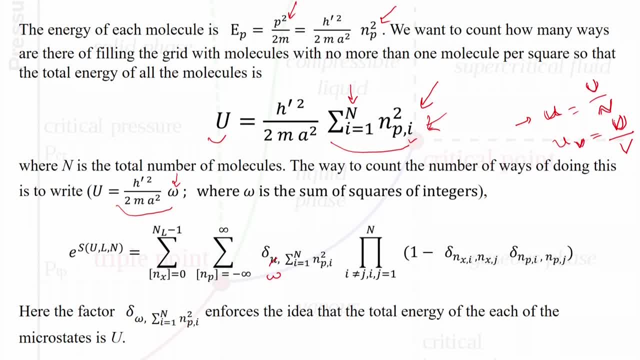 the small case u with a capital V subscript, is the energy density. that means total energy per unit volume. However, this omega is some integer which happens to be related to the total energy. So, as usual, the constraint is going to be this: that I am forced to make sure that some 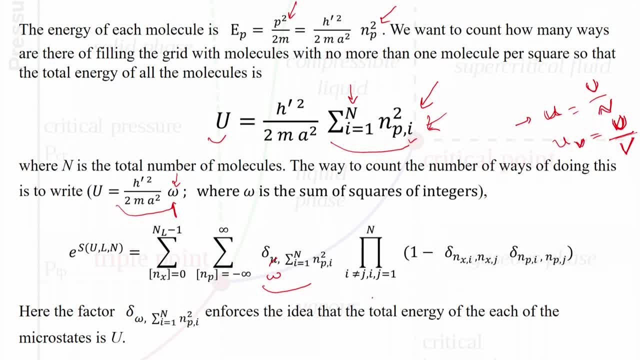 of the squares of this integer is omega. Then there is this nasty looking constraint which just tells me that only one molecule can occupy a given pixel. So that means remember there is a phase space. So I you know it is not like there is a fermion or anything. 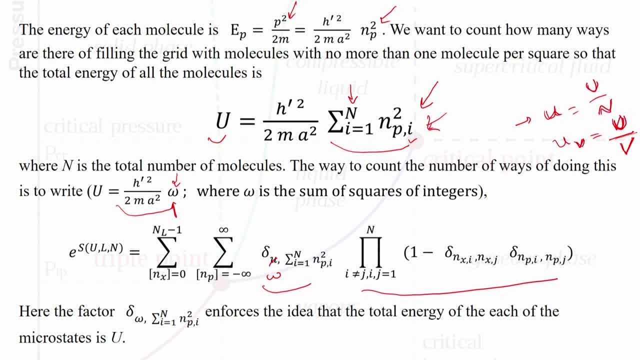 it is just that the phase space, I am going to divide my phase space into smaller and smaller pieces in such a way that I will end up with a situation where precisely one molecule is sitting in a given pixel. So in other words, suppose there are two molecules sitting in a given pixel, I divide it up. grid. 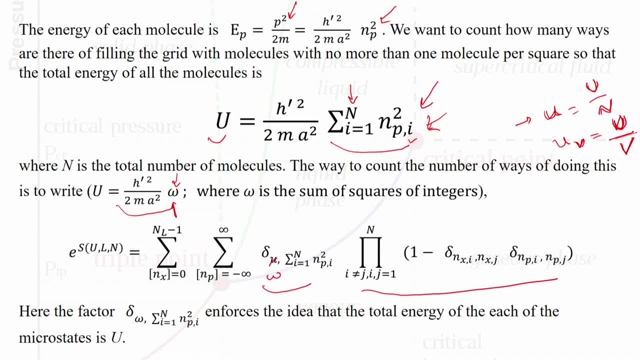 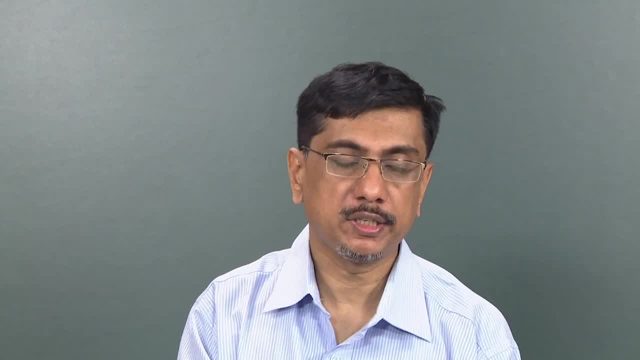 even finer. So I will make the grid even finer until I reach a state where precisely one molecule is sitting there, or no molecule is sitting there at all. So if I mean there was no molecule to begin with, no matter how fine I divide it, molecule would not suddenly. 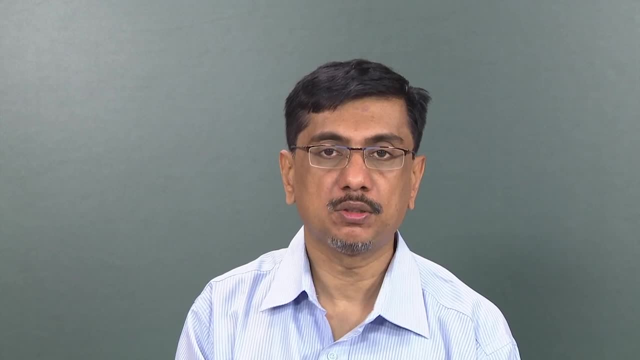 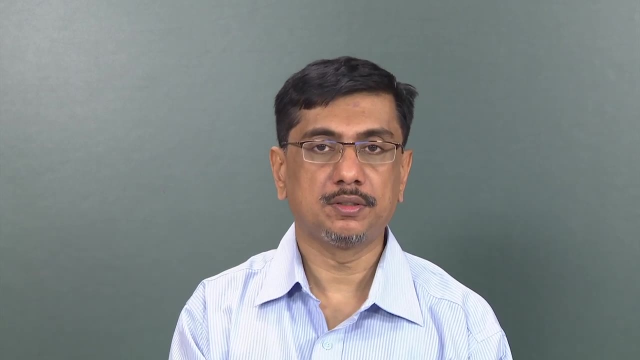 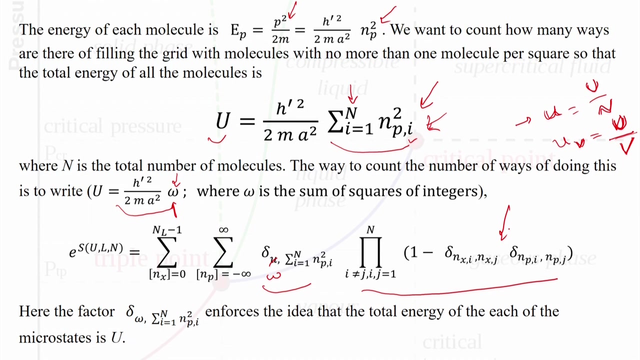 appear out of nowhere. So if it was, if two molecules were sitting, I will divide into two further. So as a result, I will end up with a grid with either no molecules or one molecule. So that is basically what this is, but this is kind of looks very scary, this whole expression. 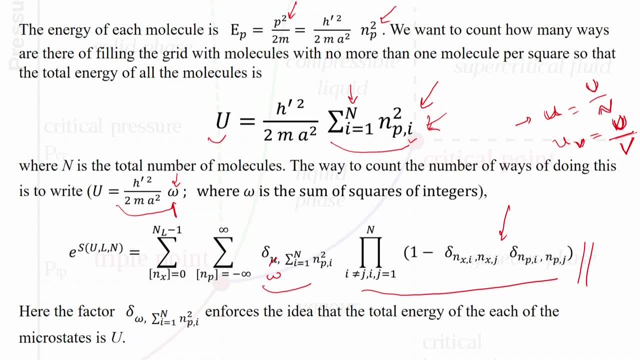 looks very scary and it is. this is how you would actually count, if you are serious about counting something which is intrinsically smooth and continuous, and you wanted to discretize it and count anyway. But fortunately we are done, But fortunately we are saved by this limit that we are going to employ, which I have already. 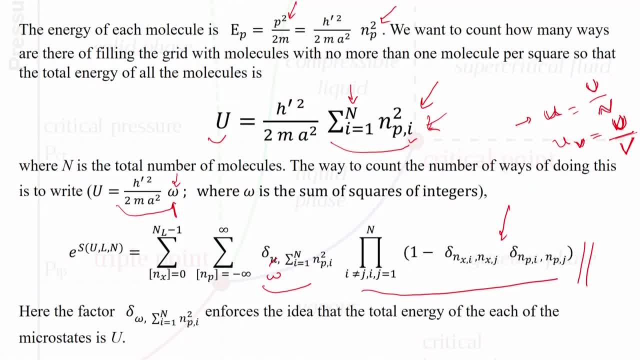 mentioned earlier and that is called the thermodynamic limit. See, in the thermodynamic limit the idea is that the total energy of the system is enormous and in fact it scales with the size of the system. So the idea is that the total energy tends to infinity. volume tends to infinity in such 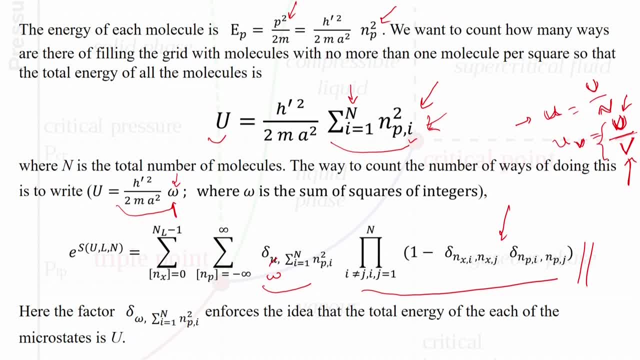 a way that the ratio is fixed. So I am going to imagine a situation where the total energy of my system is enormous. So I am going to imagine a situation where the total energy of my system is enormous. So, as a result, the implication then is like this omega, which is an integer, is an enormous 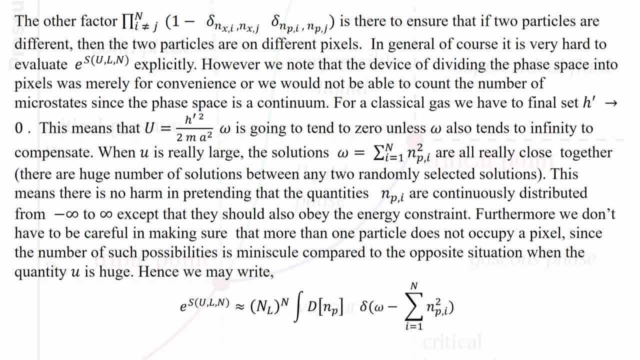 huge integer. So when it is a huge integer you can see that there will be a huge number of solutions of this. So if a certain set of integers- say np1, np2, np up to npn is an integer, then you know. 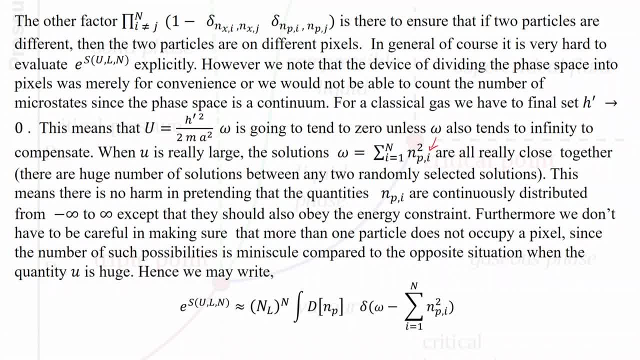 there will be whole bunch of possible solutions very close to that selected sequence of numbers. There will be a whole bunch of closely clustered solutions which are also acceptable because of the hugeness of omega. So, as a result, there is no penalty to be paid in the thermodynamic limit by replacing summation. 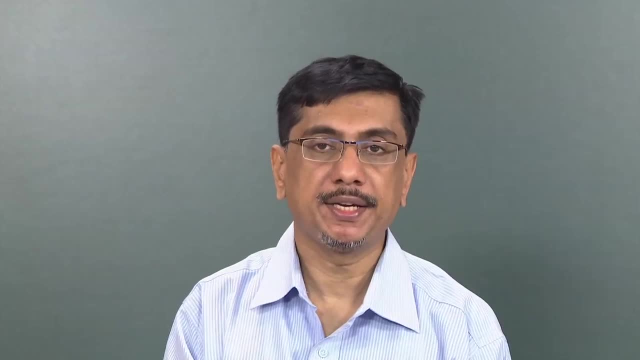 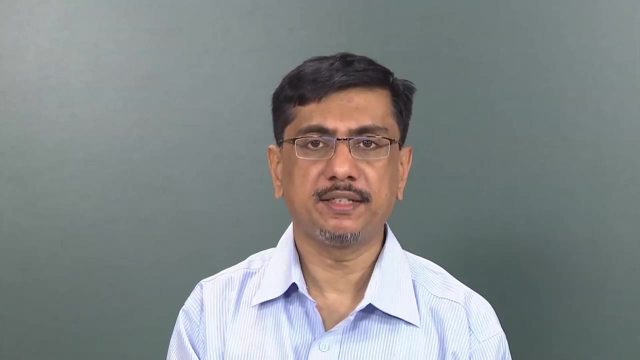 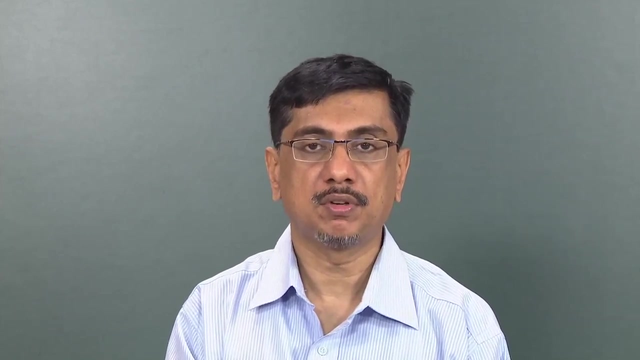 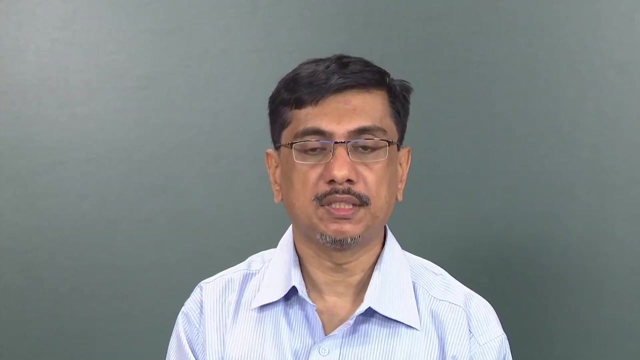 the discrete summation over these integers by an integration. So I am not going to be rigorous here and try and prove this rigorously. I did something similar earlier, if you recall, when I was trying to explain to you how to convert a discrete sum into a integration in the context of a thermodynamic limit. but here, well, this is. 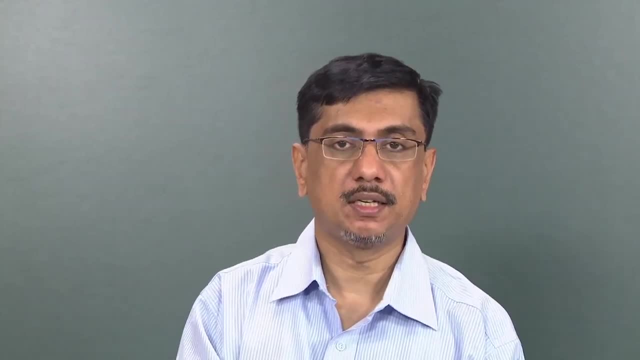 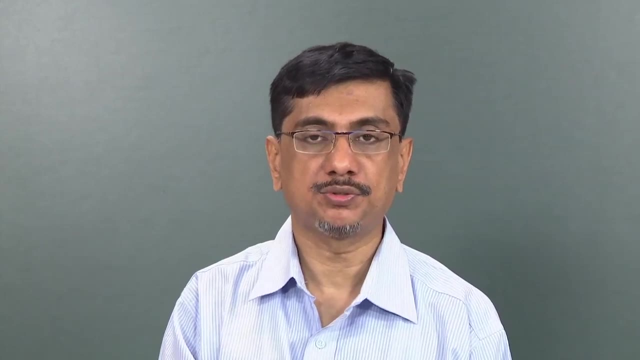 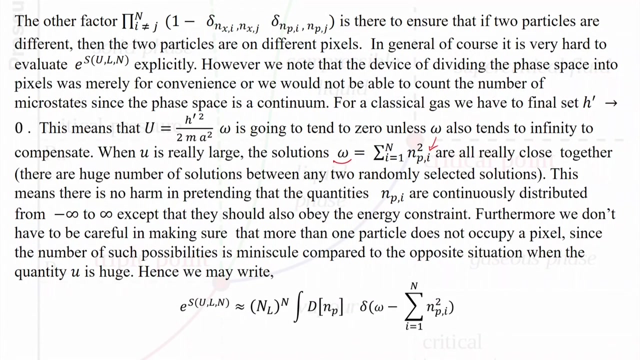 similar but not quite the same. but as a result I will either defer the proof to maybe an exercise or maybe in those of you are interested can ask me later. In any event, also the restriction Restriction that no two molecules should occupy the same pixel is also superfluous. 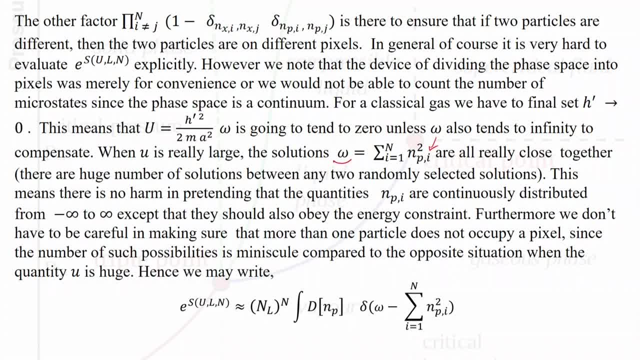 here, because in the thermodynamic limit the number of ways in which that can happen is miniscule compared to the number of ways in which the total number of ways in which you can arrange your molecules in these pixels. So it is kind of hugely suppressed the number of ways in which you can populate a pixel. 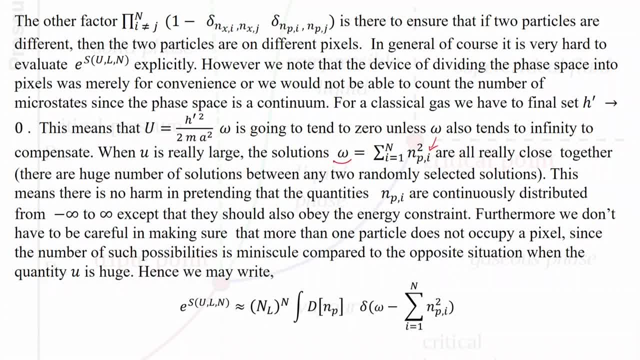 with two or more molecules. molecules is significantly less compared to the number of ways in which you can populate molecules in general, that is, if omega is huge. okay, So that is also something I will leave you to think about and, you know, come to an agreement. 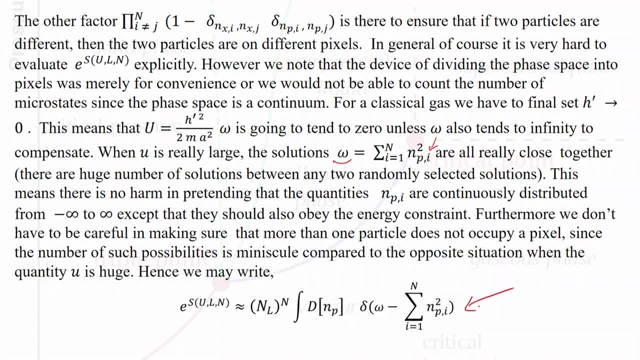 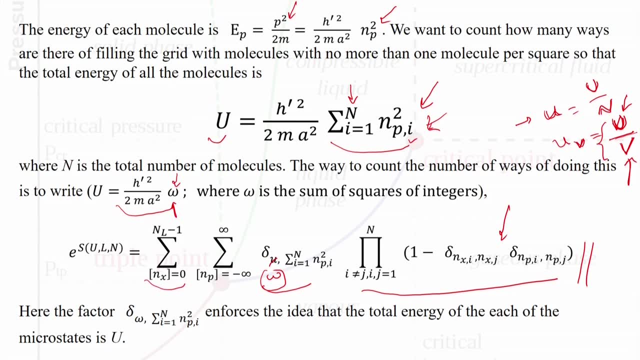 with. So, as a result, now I am in this happy situation of having replaced my summation over these Np's by integrations and notice that here, what I have here is that it is simply sum over all these discrete number of N's, Nx's, which is just counts how many steps. 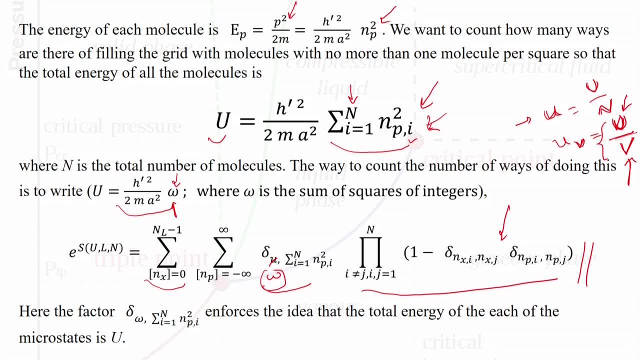 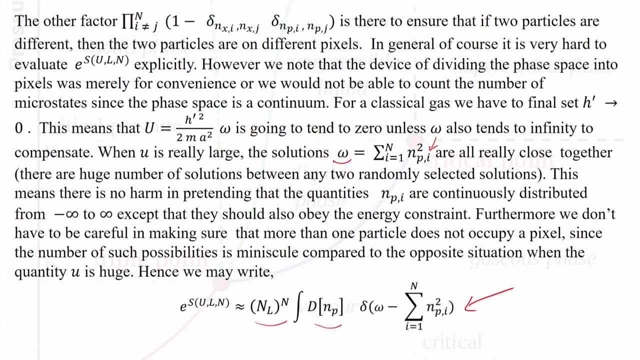 there are in the x direction. So because I have divided up my length of the box from 0 to L into NL steps, So of course you know for each particle the answer is NL, and because I have N particles it is NL times NL. So remember that I am counting the number of ways in which 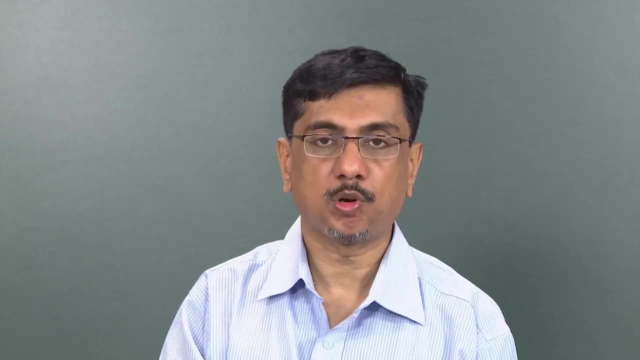 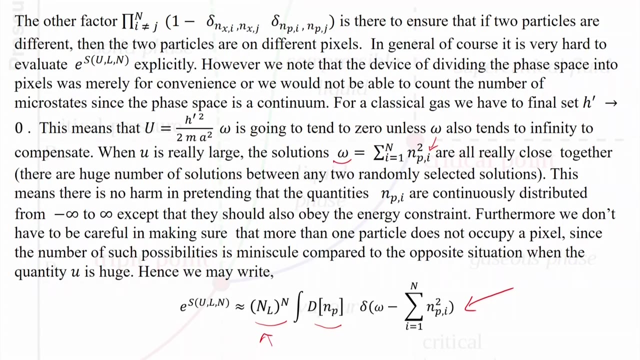 I can do things. So the number of ways is product of the number of ways of doing it for 1,, 2, 3 particles and so on. So for N particles it is answer for 1 particle raised to the number of particles. 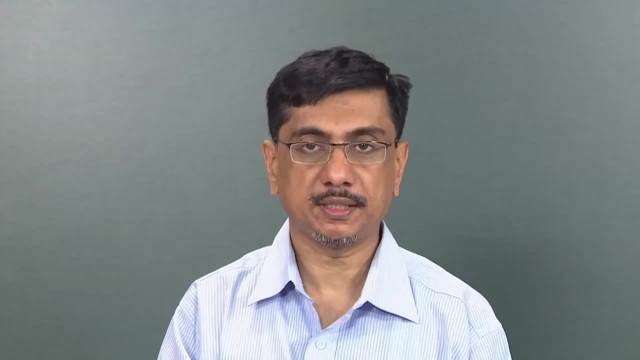 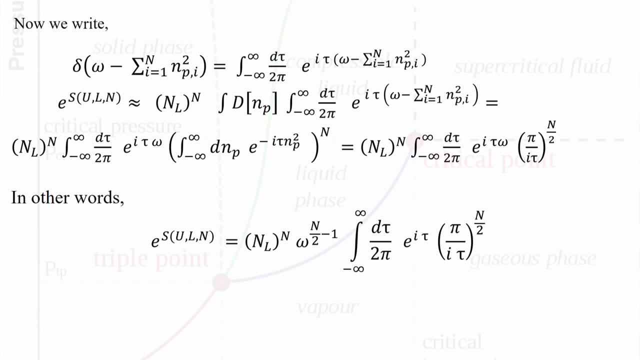 and, of course, according to Boltzmann, that is precisely the exponential of the entropy of the system. So now I am going to use my usual trick, which is to rewrite my Dirac delta function. of course, it is notice that this is not the Kronecker delta function, if it. 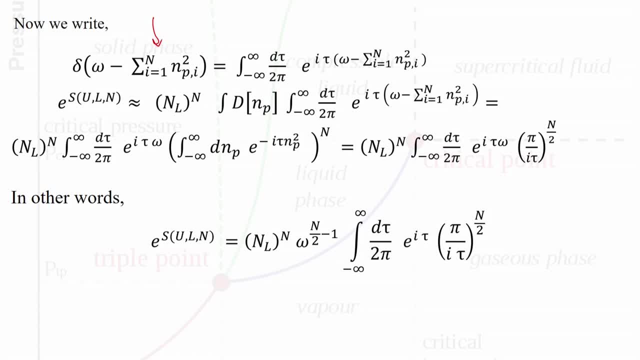 was Kronecker delta. I remember I had used angle between 0 and 2 pi. but because it is the Dirac delta I have to use a Fourier transform, So where the limits are minus infinity to infinity. So I am going to just go ahead and substitute this way of writing Dirac delta function here and then. 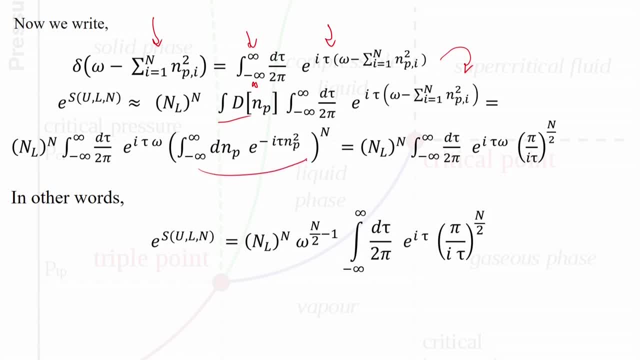 I am going to do this integral over the P's, N P's. So when I do this I end up this with this expression, And so I can extract. so you see, I am now called upon to do this integration, but I really do not care about this integration in its entirety. all I want to know is how this depends on. 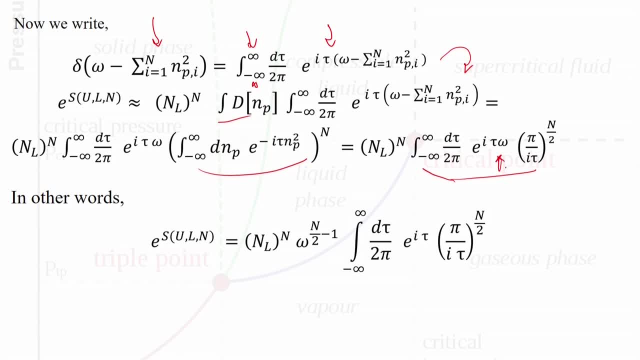 omega, which is my, you know, if you recall, omega is just that energy divided by some constant, the total energy of that system, which is huge. So I just care about how this whole thing depends on total energy, which is related to omega. So, in order to do this, what I am going to do is I am just going to rename this variable. 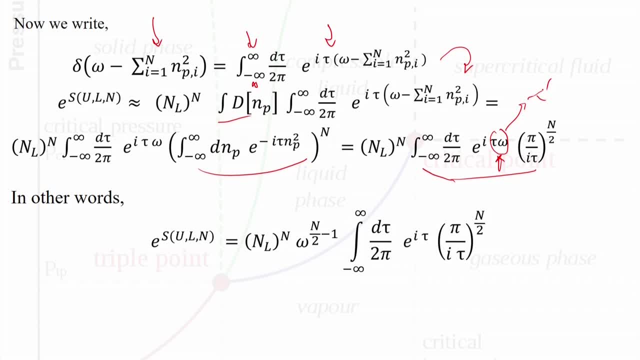 as something else, maybe tau dash. So in which case I am going to rewrite this as tau omega and then tau itself will become tau dash by omega. So when I substitute that here and also there, and then I do my integration, so actually I will get tau dash all over the 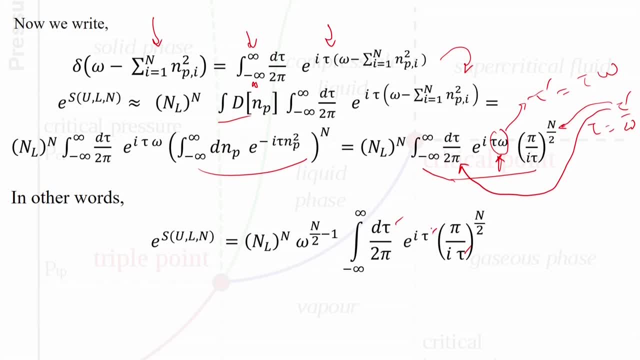 place. So basically, I end up extracting omega out of my integrations, which is all I care about. So I care about the omega dependence only, and this is just some constant. of course, this is also interesting because it depends on the number of particles, which is also of interest. 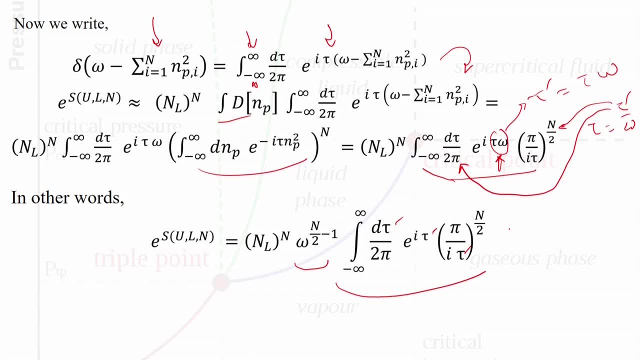 in some sense So, but nevertheless, this is the answer And I can now go ahead and use my tables. or you know some software. my preferred software is called Mathematica. Well, I am not a spokesperson for this company, Wolfram Mathematica, I just happen to use it. you know, I do not have shares in this company, so I am not advertising this. 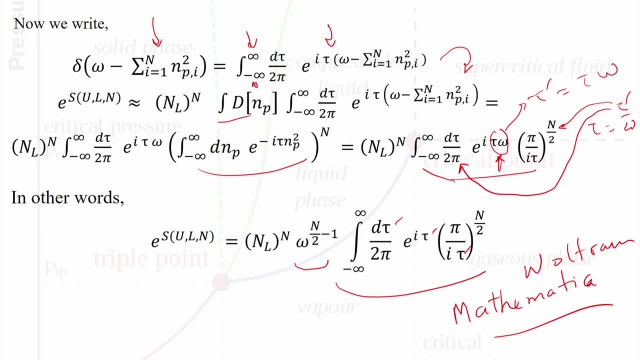 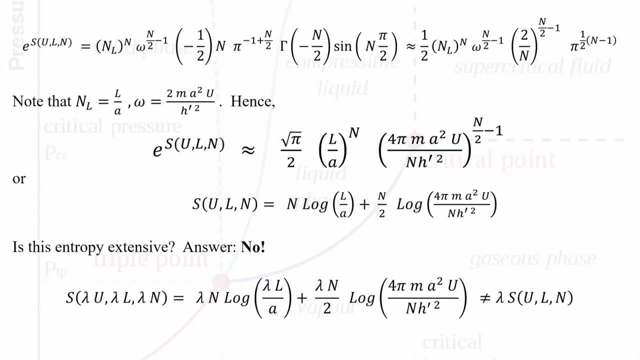 but there are other products that are used also. they are equally useful- Matlab and so many others- So you can go ahead and use that and perform this integration and you end up getting something like this and in the end, result is this: So now I am going to go ahead and bring back 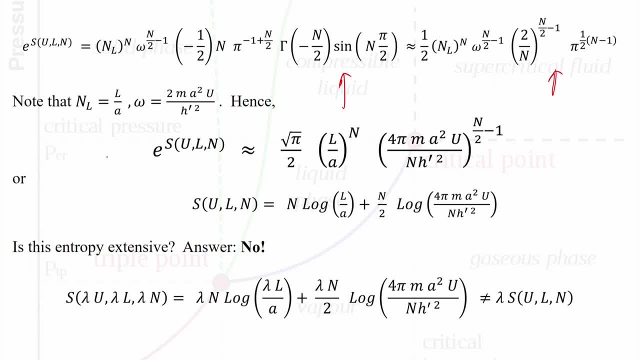 the quantities that I was started off with, namely the length of the system and also the total energy of the system. So let me bring that back. So when I bring that back, the exponential of the entropy, It is going to start looking familiar. so it involves total internal energy number of particles. 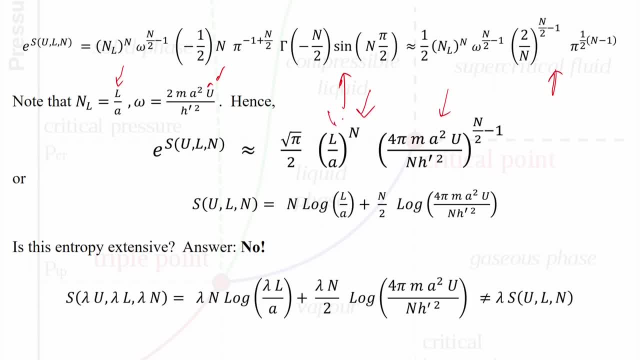 and the size of the system, L. okay, So now I take the logarithm of this and I end up getting this. So now the important question that I have to ask myself is this entropy function that I have derived, which is a function of the total energy U. 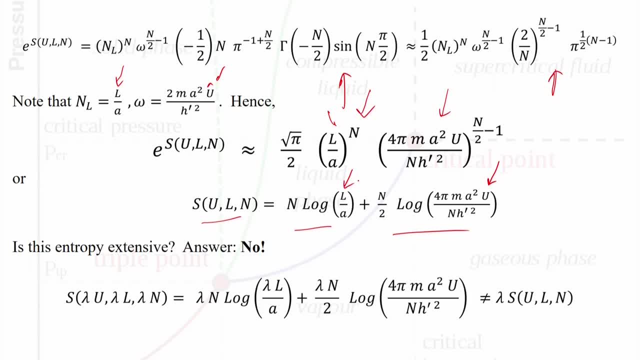 The length of the system- Okay, Length of the system L and the number of particles N? is it extensive? So recall that an extensive function is one which has this property, namely if you take S of U, L, N and I balloon each of these quantities by a factor lambda. 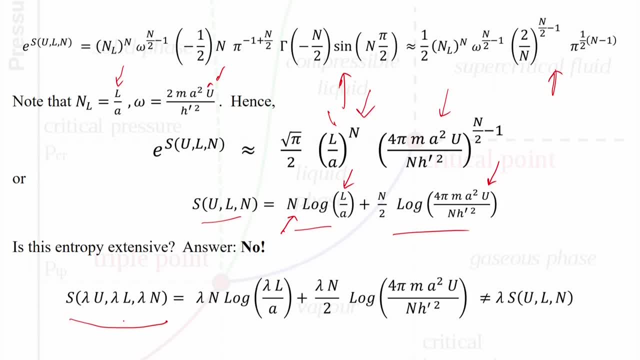 So in. as a result, my U is replaced by lambda U, L is replaced by lambda L and N is replaced by lambda N, and if S was, were extensive, it should become lambda times S of U L N. So if that is, if S were extensive. but now let me stare at this answer and ask myself: does? 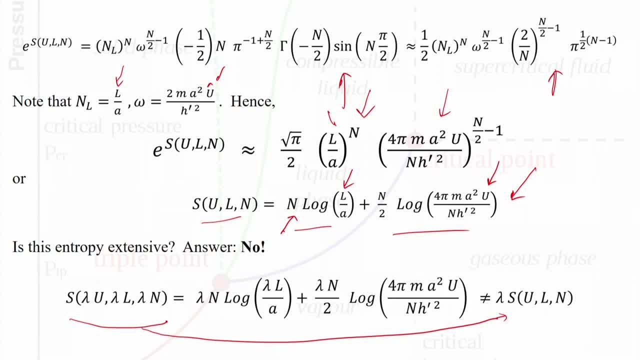 it obey this property of extensivity? The answer is no, because of this reason that of course this lambda comes outside here and there, but then it goes away here, because if I scale U by lambda, Okay, I scale N by lambda, then lambda cancels out, as it should, but however, there is nothing. 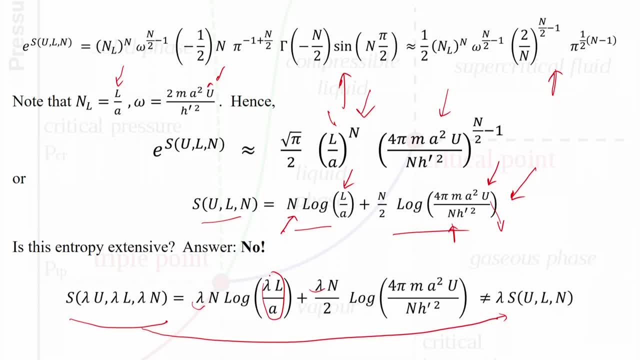 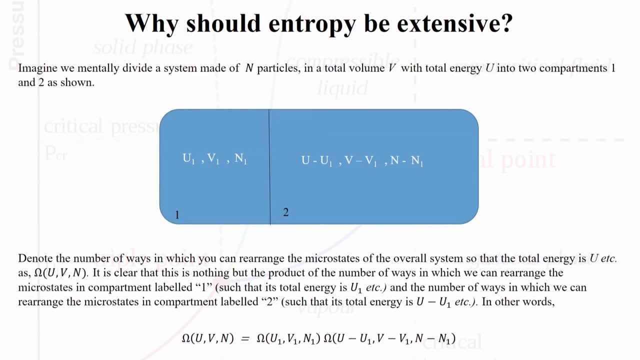 here to cancel the lambda. So there is a lambda that remains in the log. Okay, So this is annoying because I want entropy to be extensive. So the question now is, why should entropy be extensive? So let me try and answer that question. So this is important. So the reason 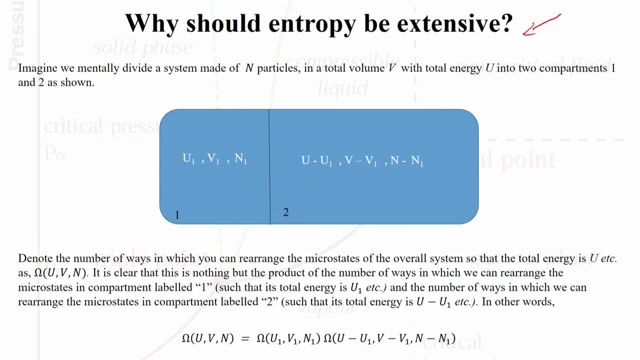 why entropy should be extensive is if it is not extensive, If it is not extensive, it kind of leads to an uncomfortable paradox. So imagine that there is a huge system of, say, let us talk about a gas right now, So which has a total internal energy of U and total volume of V and total number of particles N. So imagine, 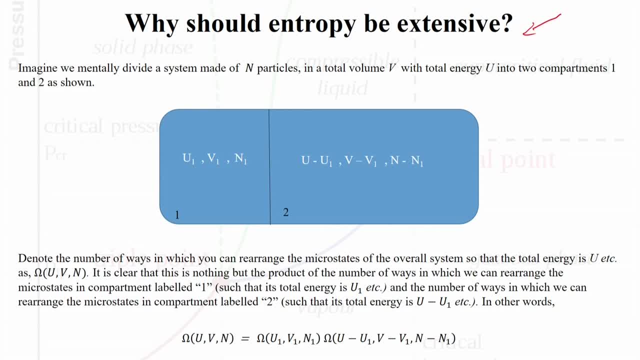 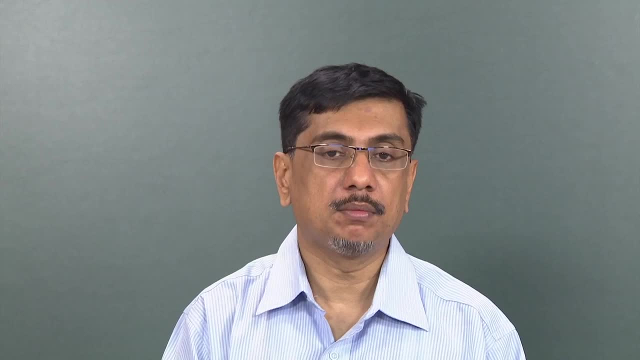 I kind of mentally partition this into two pieces. So Pv has U1, N1- or yeah, N1- number of particles and V1 volume and the other has a remaining energy volume and number of particles. So clearly the number of ways I can rearrange. 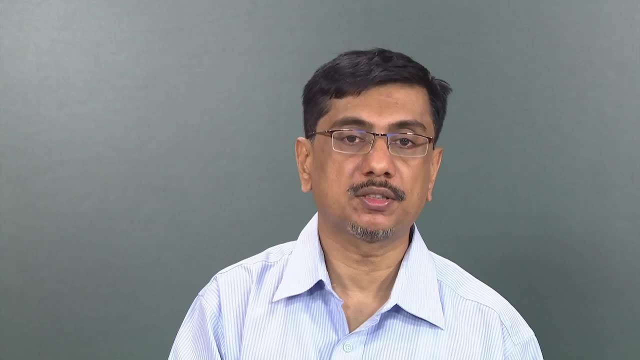 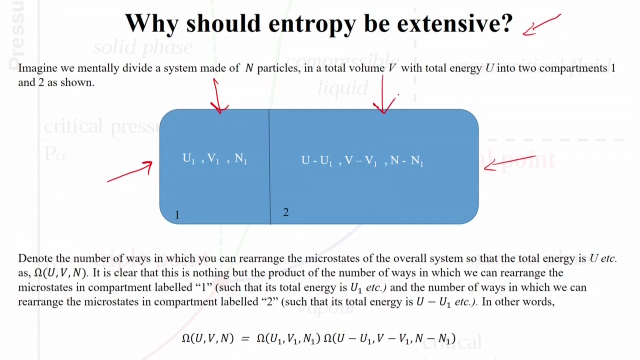 the microstates of the combined system is simply the product of the number of ways in which I can rearrange the microstates of this mentally partitioned subsystem and the way in which I can rearrange the microstates of the second partition. So that is what I have. 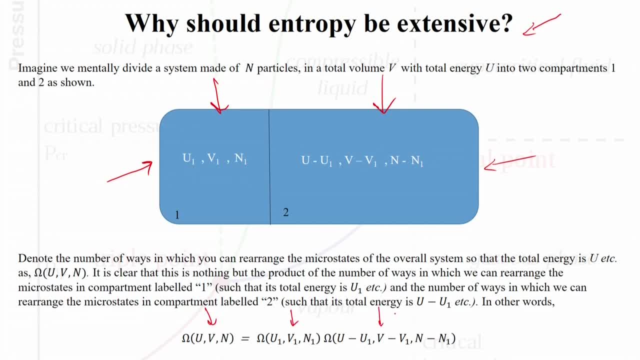 written here. so I expect this to be the case. Now I can show you that this is nothing but the statement of extensivity of entropy, because I can remember that omega is nothing but the exponential of the entropy of the system. So, as a result, I take logarithm on both sides. 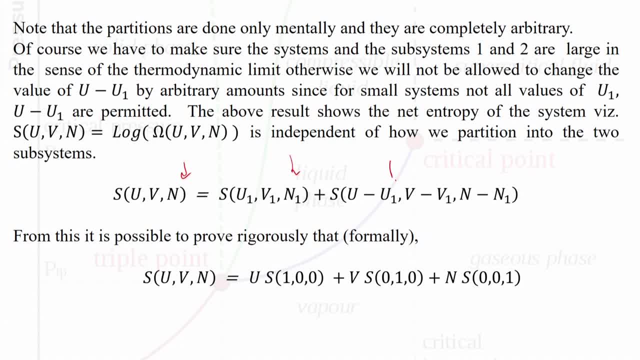 I end up with this equation, okay, So now you can show. we will probably relegate this to some tutorial or some other exercises, So you can show that the only answer that is consistent with this equation. remember that I can partition this. there is no restriction on u1, v1 and n1, of course, the only restriction. 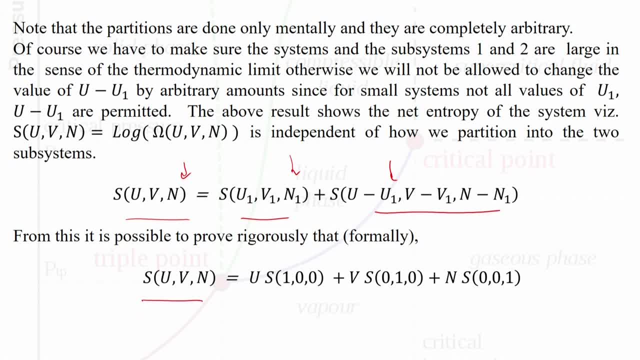 is that these u and v have to be very huge, otherwise I cannot really strictly speaking. if u and v and n are not huge, Then I do not have any right to kind of mentally partition it in some random arbitrary way, because you know then I will not be able to have solutions of those Diophantine equation. 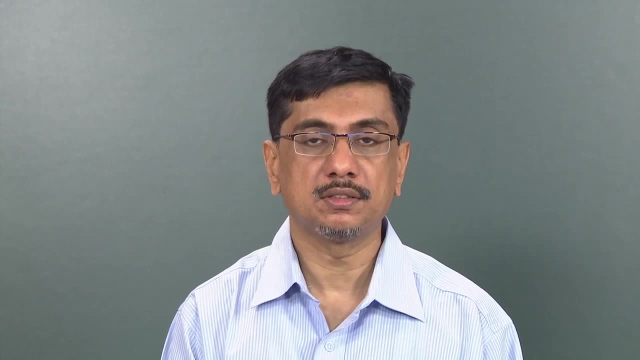 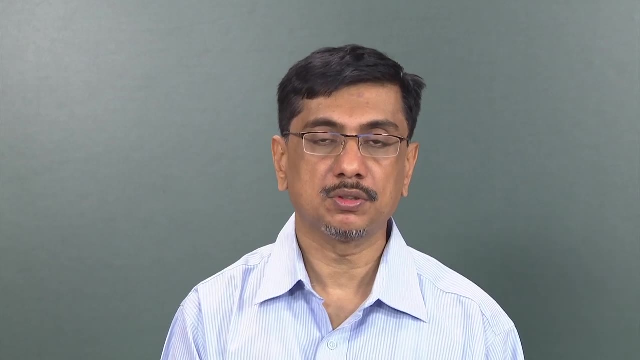 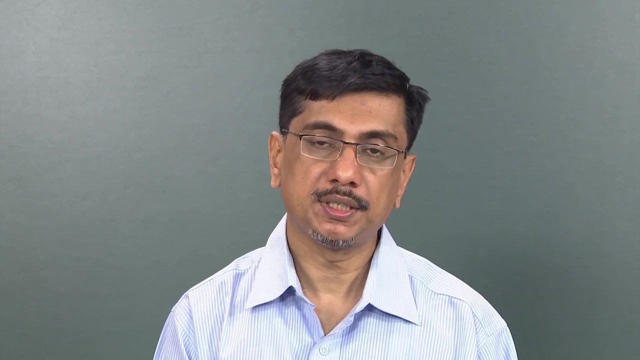 you know willingly, So I will have to. only certain kind of partitioning will allow solutions and certain other kind of partitioning will give me no solutions at all. However, if these u's and v's are huge, then I am kind of at liberty to partition. 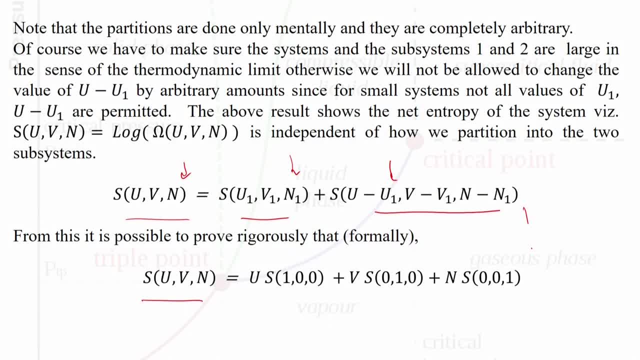 It any way I want, so you can convince yourself in the exercises that the only solution consistent with this equation is the solution which makes S extensive. so that means it is linear in u, linear in v and linear in n. So now the uncomfortable paradox that we have in front. 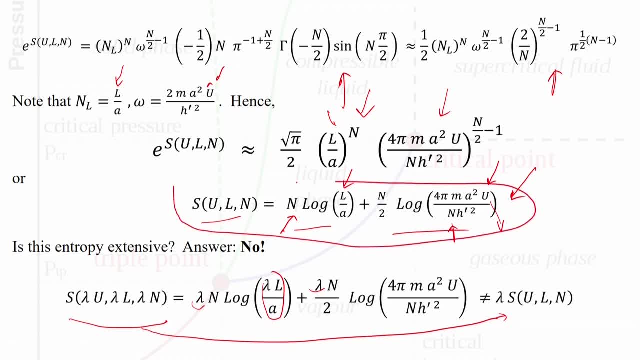 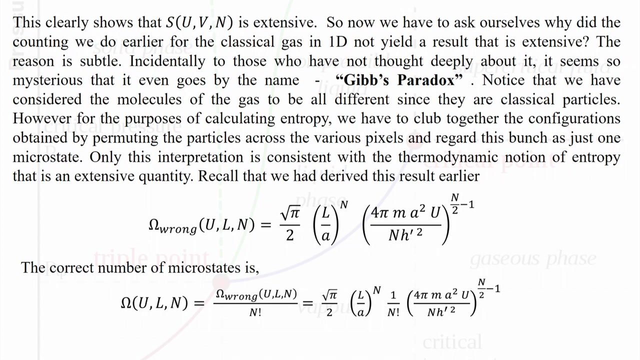 of us is that we seem to have done this correctly. we have counted the number of microstates by partitioning the phase space into small grains, small pixels, and yet we are unable to come up with an expression which is extensive. So this is known as Gibbs paradox. so Gibbs not only stated the paradox, but also gave. 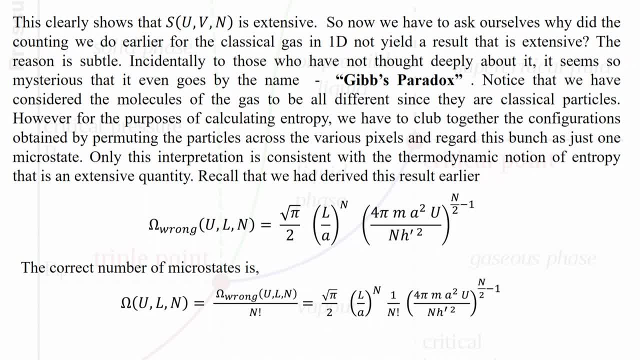 a solution. so, instinctively, what we have done basically is we have thought of all the molecules as being different. So basically, what we should do is that if I take, say suppose, there is one molecule occupying this pixel and then there is empty pixel, empty pixel, then there is another molecule occupying 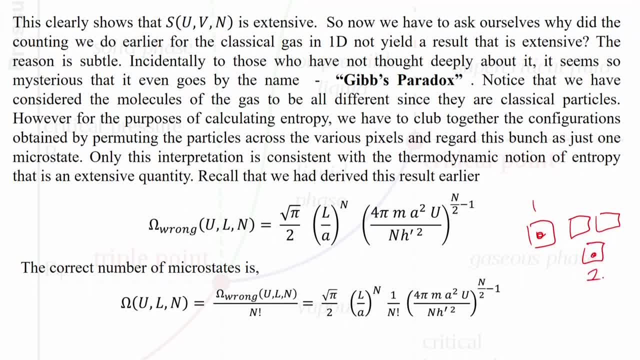 this pixel, So I call this. what I have done, instinctively, is I have called this molecule 1 and molecule 2, and I have considered these two states as being different. okay, So what I have done is I have considered this to be different. 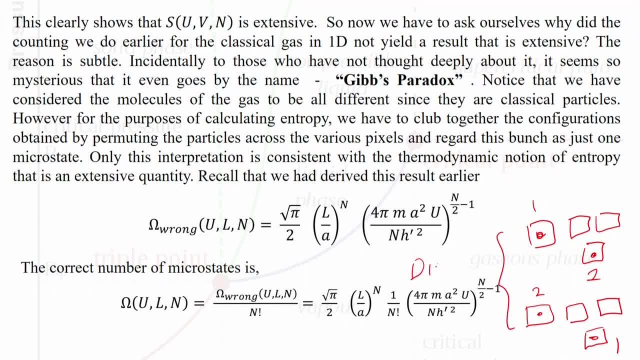 So I have considered these two to be different while counting. So just think about it. So that is what I have done, But what this paradox is suggesting is that I really should not have done this. so, in other words, it is telling me that I had better not consider these two. 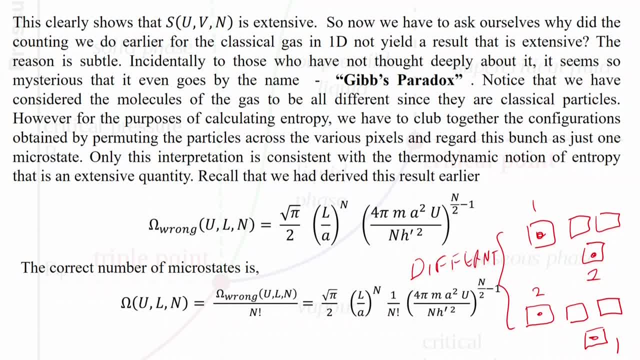 configurations as being differentSo if the molecules are all identical, I am compelled by thermodynamic necessity divide by a certain factor of n factorial, which is basically the number of ways in which I can permute in all the molecules which are occupying these pixels. So this is the only. 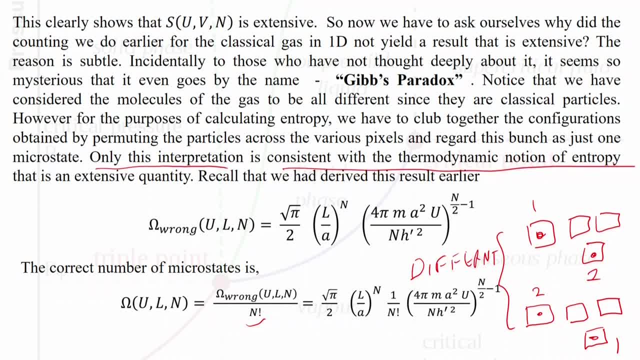 interpretation that is consistent with the thermodynamic notion of entropy. that is an extensive quantity. So I would not really try, and you know, derive this in any more convincing way, because I do not think there is such a derivation. it is just so happens that if you 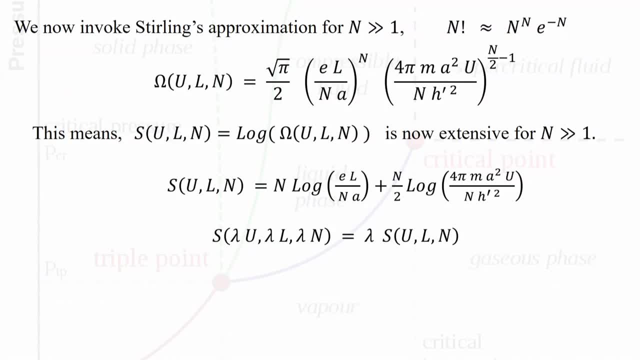 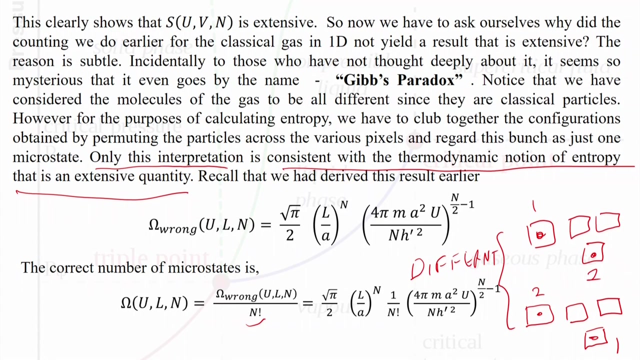 do this, you get an entropy that is extensive. So now how do I show that is because use Sterling's approximation. So recall that when n is huge, n factorial is approximately n raise to n times e raise to – n Again. you are supposed to know all this from some math course maybe. So just go ahead and substitute that here. 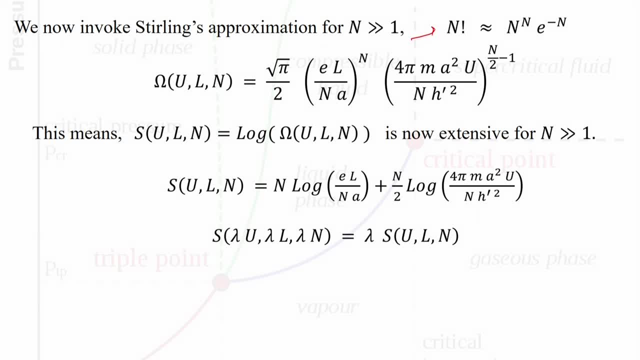 and let us see, And lo and behold, you get an expression of this sort where L gets divided by n, which is an intensive quantity- and this is anyway, it was already an intensive quantity- raise to n by 2.. So now, if I take the logarithm of omega, which is my entropy, I get a happy 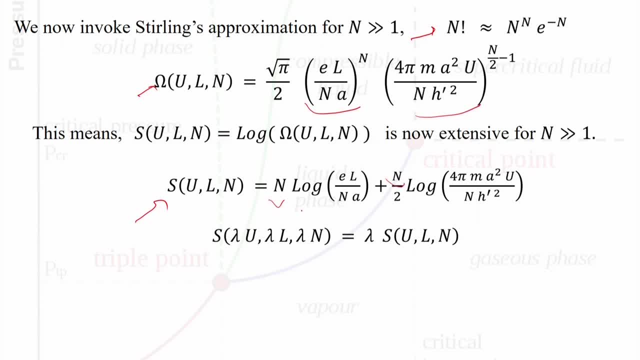 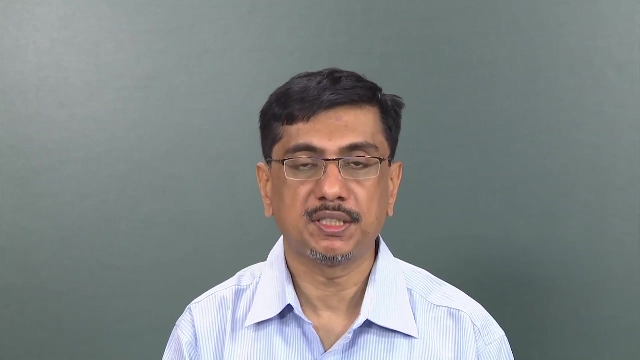 result, which is proportional to n, and proportionality factors are intensive quantities. So now this will certainly Extensivity, and this is what I was looking for. So notice that I have restricted myself till now, just for simplicity, you know. I just wanted to learn how to count phase space when. 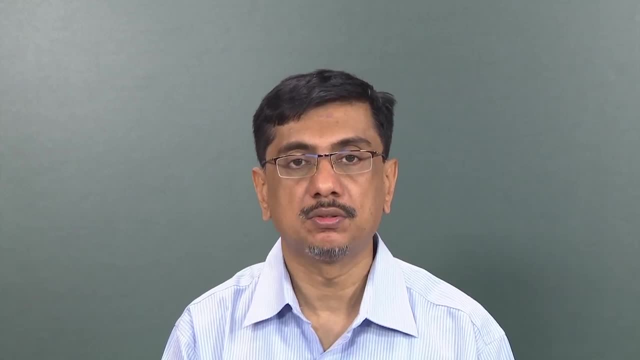 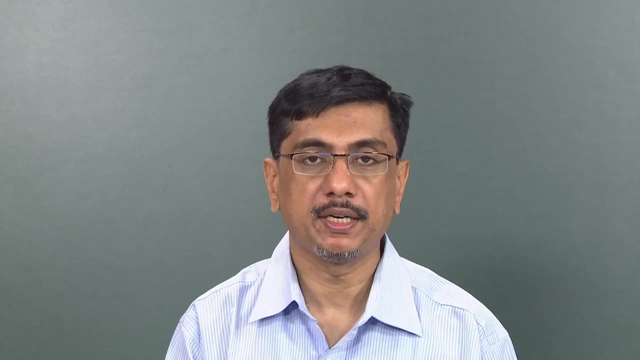 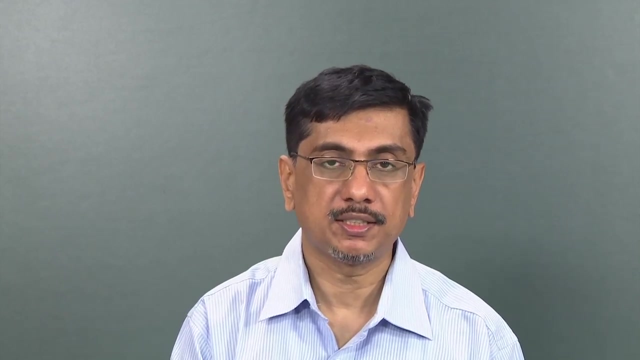 you know, by discretizing it into pixels. So I, as a result, restricted it to one dimension, because I already have two quantities, which is momentum and position, and I cannot afford to draw a picture on a flat sheet of paper if I go beyond one dimension, because I already 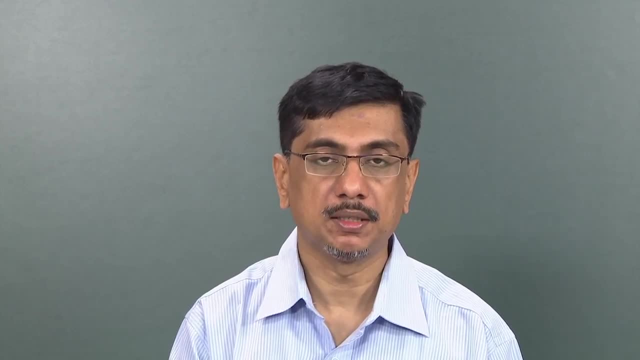 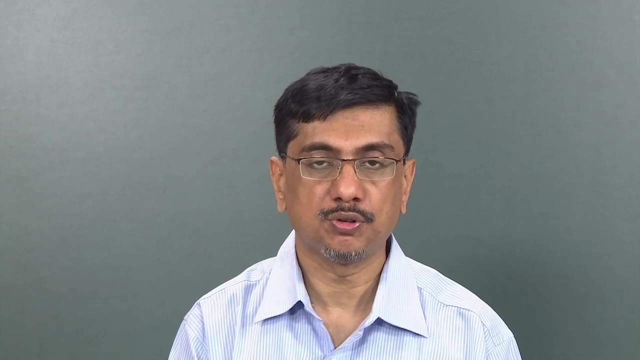 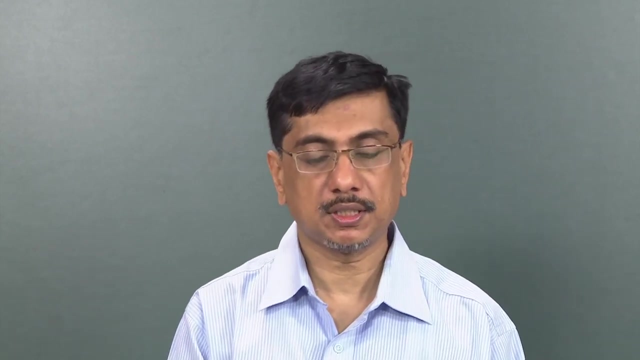 have two there. So I mean position and momentum, and then I have. if I have more than one position, then I will have to immediately go to four dimensions, because I will have two positions and two momentum components. So that is the reason why I was restricted to look at one. 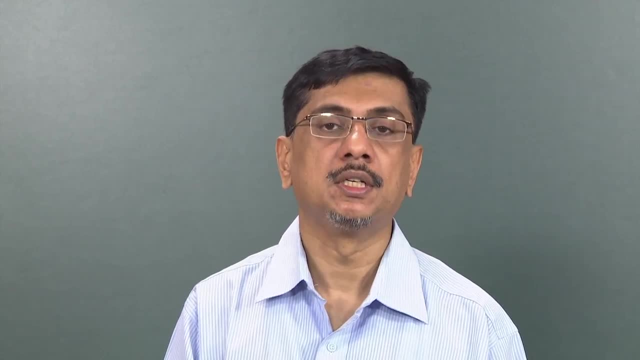 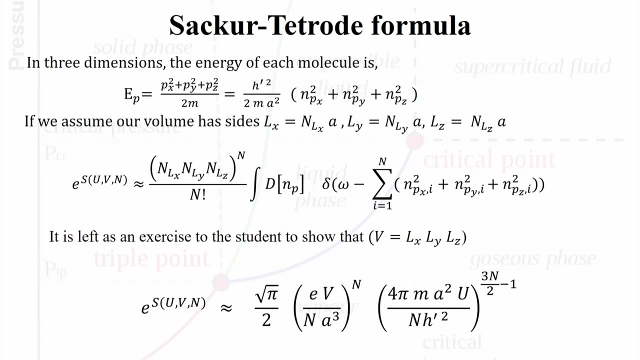 dimensional molecules in one dimension. So now let me use my mathematical imagination and see if I can generalize this to what is physically the case, which is a three dimensional classical ideal guess. So in that case I have three components corresponding to x, y and z. So for a given molecule, already there are: 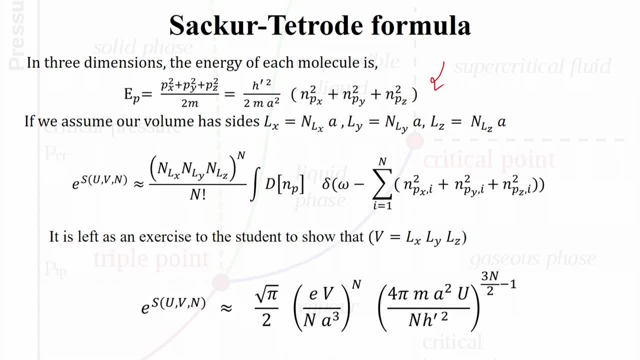 going to be three integers: npx, ny and npz. Well, this is less important. this is clear what is happening here. So it is just volume. So I am going to write this as x and z. So clearly there are three directions, So, but what is really interesting is this one. So 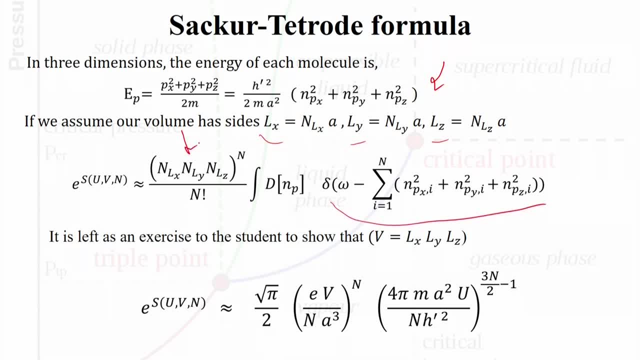 I am going to have to do this carefully. This is obvious. So you have so, in the x direction, raise to n. y direction, raise to n, z direction, raise to n. And of course this is my Gibbs factor which prevents the paradox from happening. and of course, even here, if I am, if I do not, 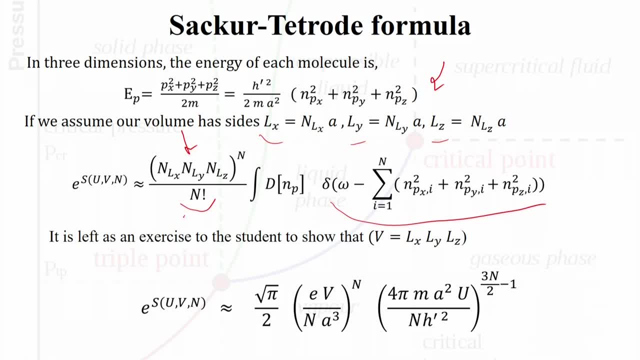 put this, I get a paradox, which, in other words, the entropy is not going to be extensive. But what is really important is that I have to learn how to do it in three directions. So I am going to have to do this carefully. So you have. so, in the x direction, raise to. 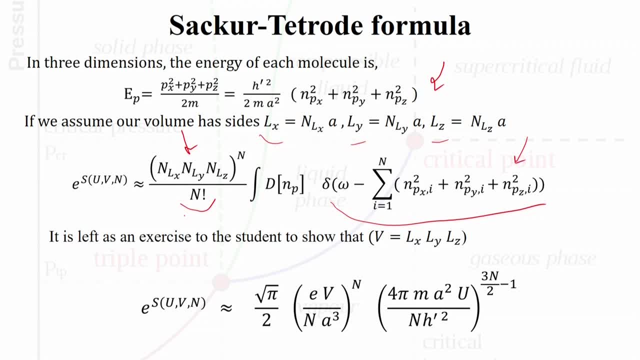 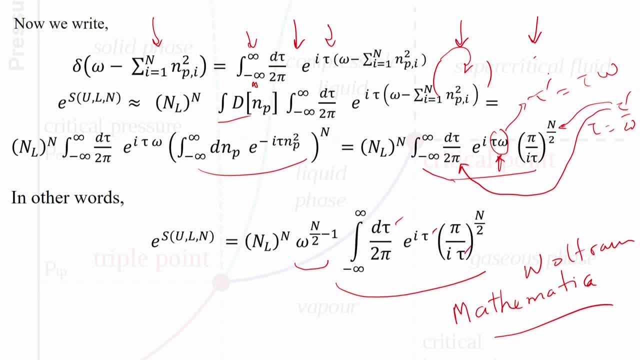 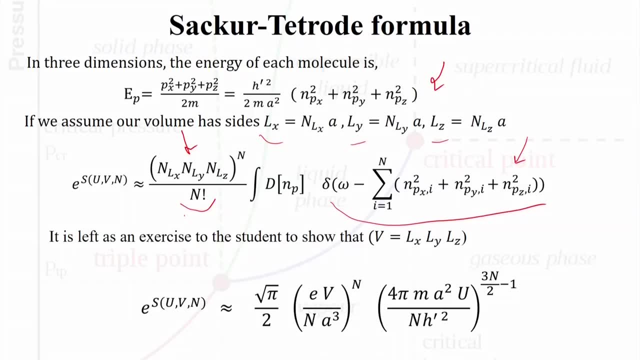 this thrice, once, twice thrice. similar thing for n, x, n, y. So I will end up getting you know three copies of the same thing, okay? Well, it is slightly more complicated than that, but it is roughly that, okay. So I mean, it may not be exactly that. That is why I have written. it is left as an exercise to